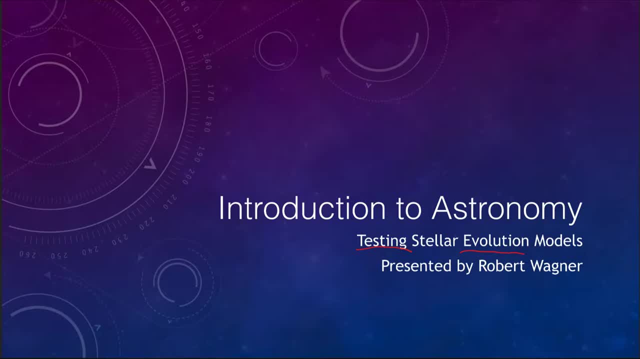 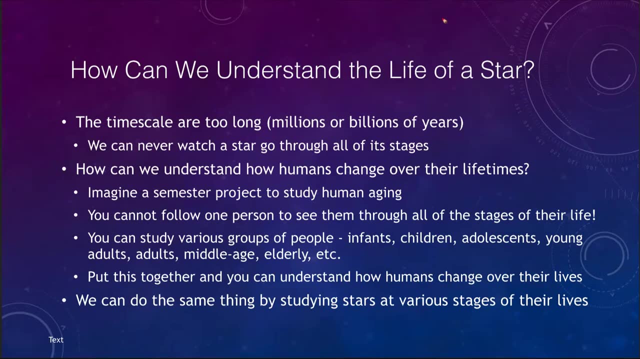 stellar evolution work. So let's take a look at this and get some ideas of it. First of all, first thing we want to look at is how can we possibly understand the life of a star? What we have to think about is that the time scales are minimally millions of years and more likely for stars like 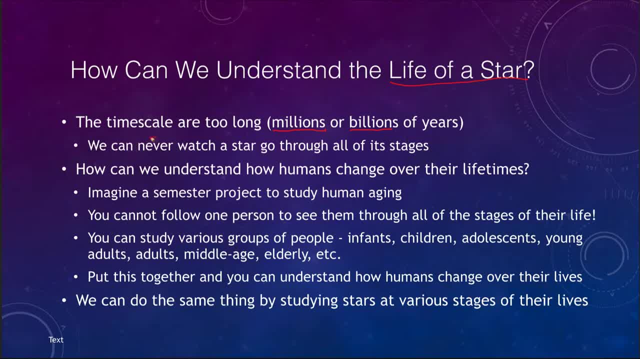 the sun billions of years, meaning that we can never watch a star go through all its stages of life. We cannot watch one star, even over multiple human lifetimes, go through all of its stages. In fact, even over multiple human lifetimes, stars are unlikely to change at all. So one way that we can 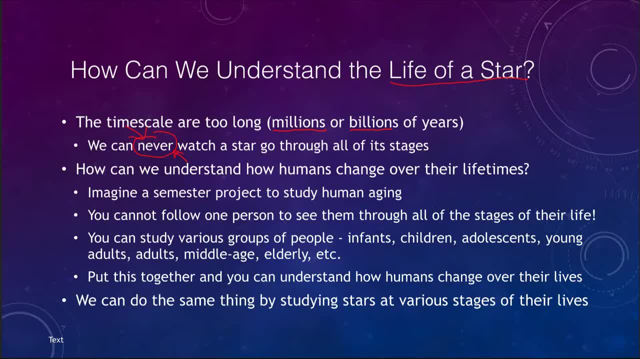 look at this and try to understand how we can understand stars even though we can't watch an individual star go through its life. is that how can we understand how humans might change over their lifetimes? And you can imagine a semester project to study human aging. Well, in a semester you cannot follow one person. 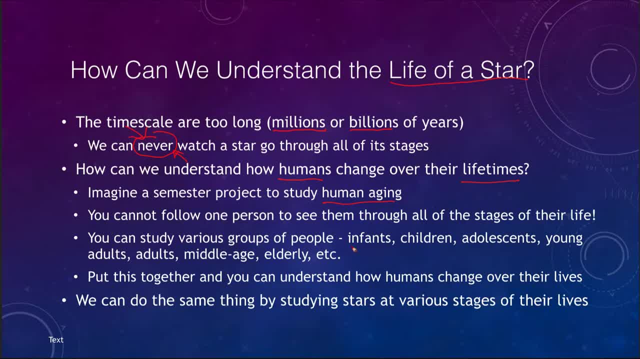 through all the stages of their life. But you can study all different stages, from infants, children, adolescents, young adults, adults, middle age, elderly and so on. You can study all those various different groups and put this together and you could still be able to understand how humans do change over their 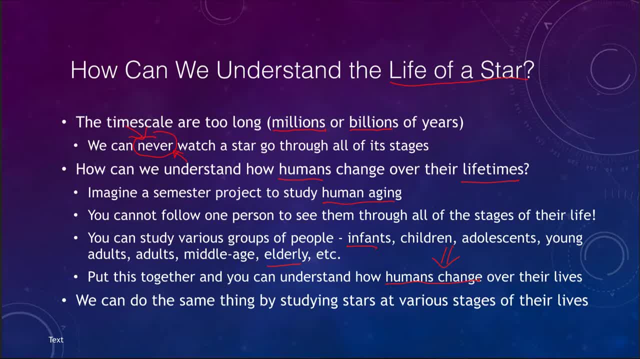 lifetime, Even without studying just one human and watching one human change their lives. Well, we can do the same thing with stars. We can look at stars at various stages of their lives and then use that to be able to better understand the life cycle of a star. 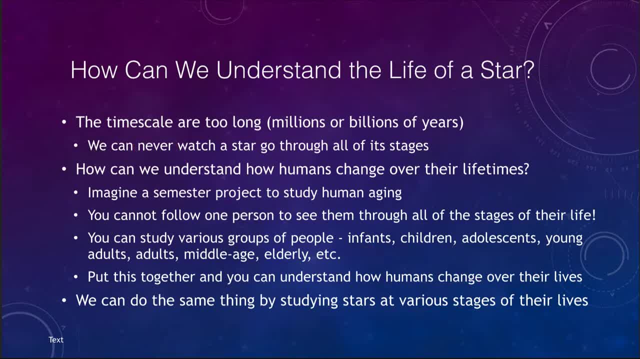 So let's take a look at some of one of the ways that were able to do this, and one way that we can do this is using star clusters. Star clusters are very highly significant. It's extremely important to understand how stars work, and the very same way that we can do this- and one way that we can do this- is using 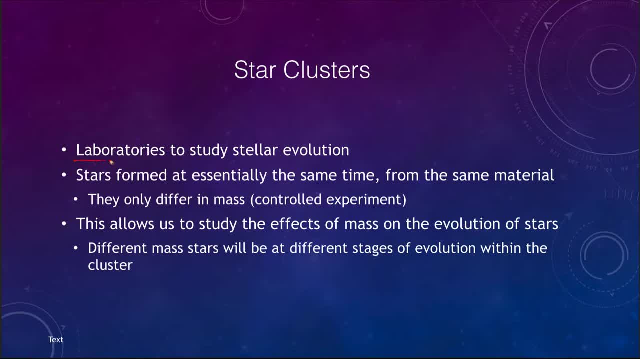 star clusters. Star clusters are dependent on each other. Star clusters are essentially laboratories that we can use to study the evolution of stars. The reason they are such good laboratories is that the stars in a cluster formed at essentially the same time from the same material. 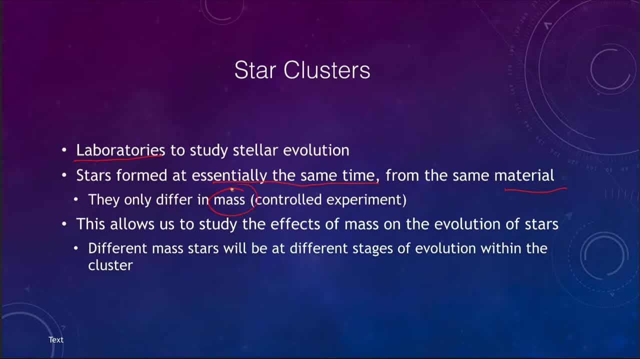 They differ only in one thing: They only differ in their mass. how much material formed each individual star? Think of this as a controlled experiment. If we just look at random stars in the sky, they could have formed at different times. The materials could have been slightly different. 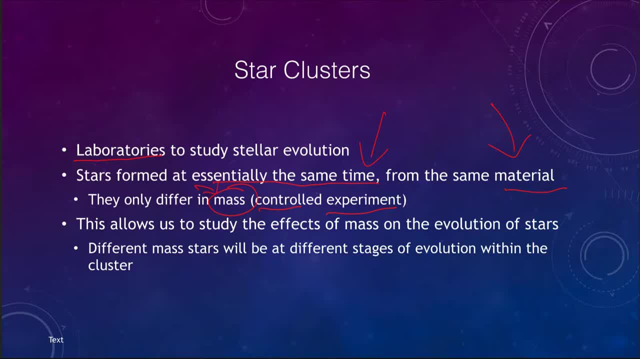 And their masses could have been different. We're not able to look at just one variable. This can be a controlled experiment in which the times and the materials are the same, So now our only difference is the masses. So it allows us to study the effects of mass. 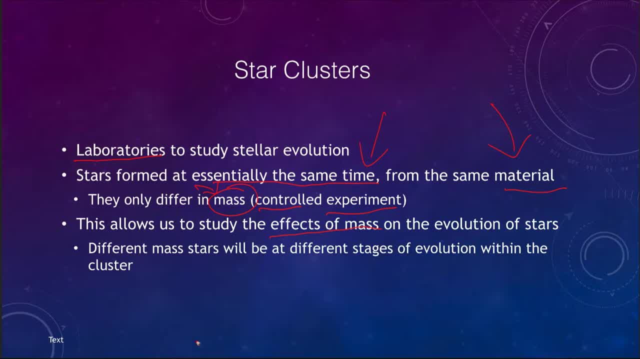 on stellar evolution And what we find is that different mass stars will be at different stages of evolution. Remember that high mass stars evolve very quickly, taking only millions of years. Low mass stars can take billions or even trillions of years to evolve. 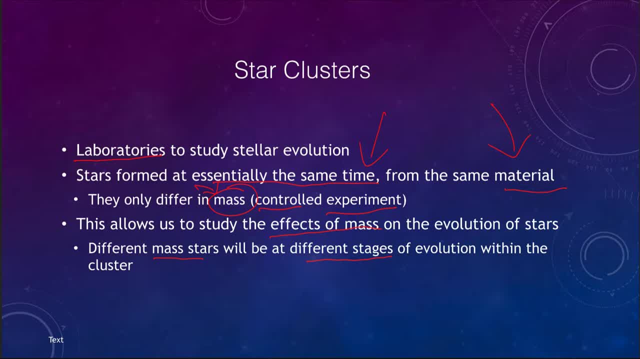 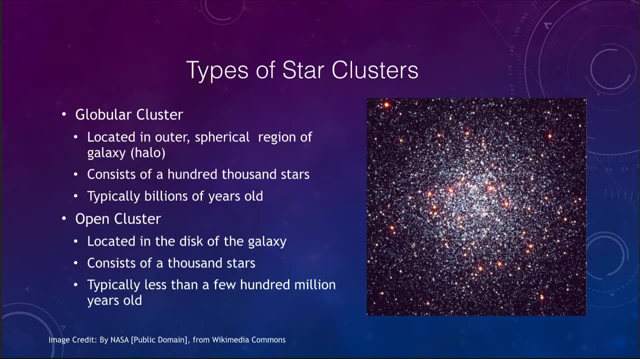 So we can see all of those different stages at different cycles in a cluster. So let's look at an example and see what these clusters are like. First of all, there are a couple of different types of clusters that we want to look at. 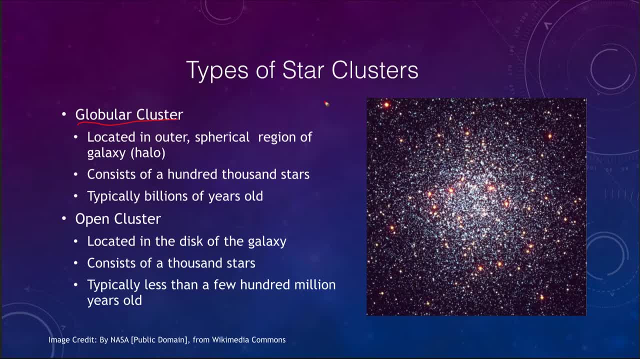 And one type is what we call a globular cluster, which is pictured here. These are located in the outer region of our galaxy, which we call the halo, the spherical region of our galaxy. They can contain hundreds of thousands of stars and are typically many billions of years old. 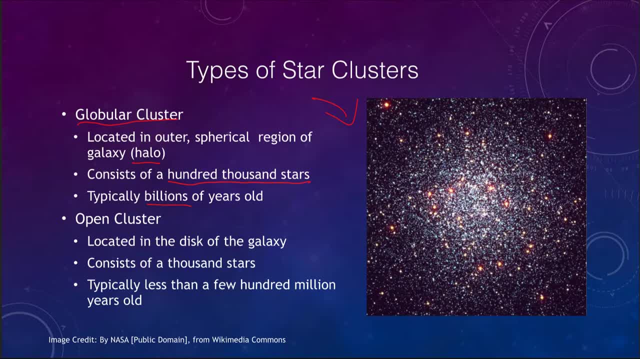 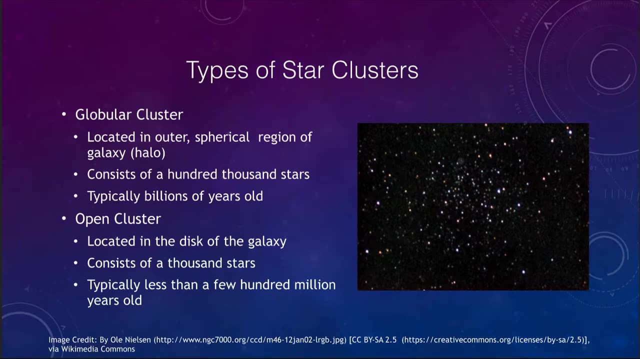 So these are very old clusters that have been around for a while, And there are other types of clusters that we can look at, which are much younger clusters, And these are what we call the open clusters. So an open cluster by comparison. 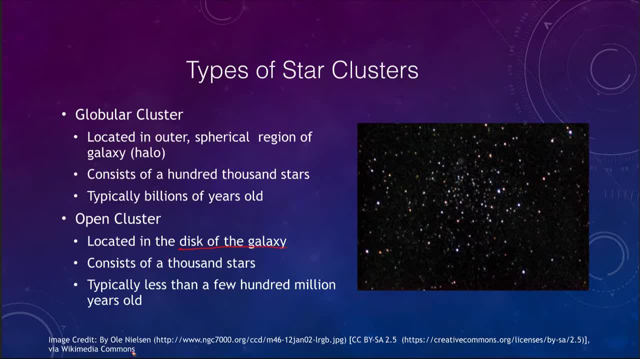 is located in the disk of our galaxy, so in the flattened portion of our galaxy. They may only contain several thousands of stars And they're typically less than a few hundred million years old. So an open cluster here, as we can see by comparison. 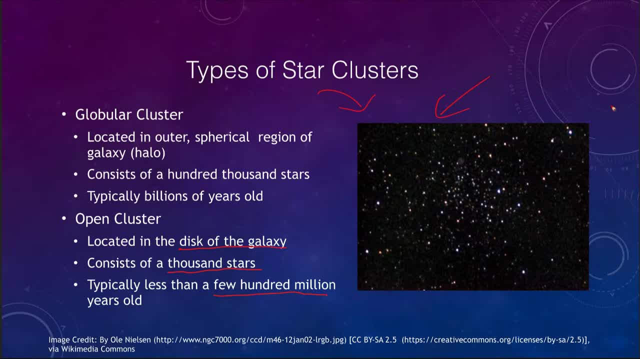 is much more spread out than the globular cluster that we looked at previously. Fewer stars Has a lot of stars, A lot of younger stars, And they are more spread out. An open cluster will eventually dissipate out into space, whereas a globular cluster has enough material. 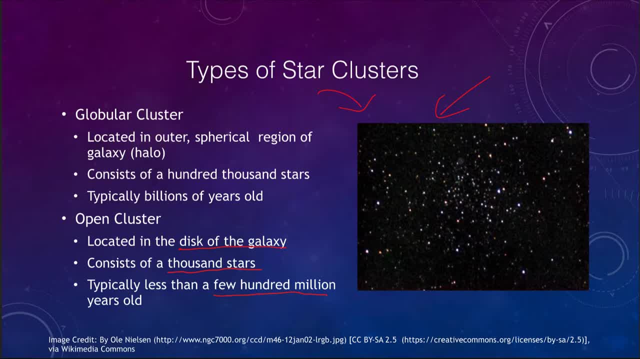 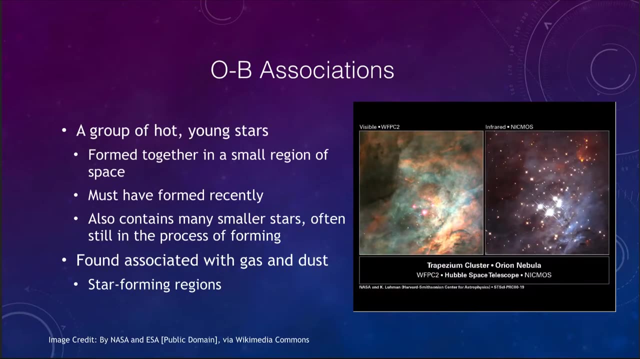 there to remain bound together for billions of years. So one other type that we can look at is what we call the OB associations. These are even younger than the young open clusters. This is a group of very hot young stars that have formed together. 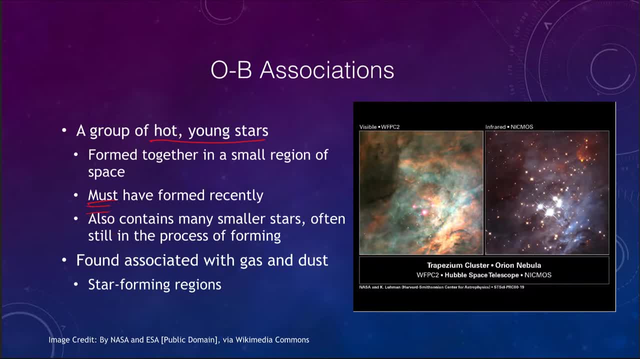 And we know that they must have formed recently, because they contain stars that only live a million years, or sometimes even less. So they must have formed very recently, Otherwise those stars would not still be here. However, they also form many smaller stars, so low mass. 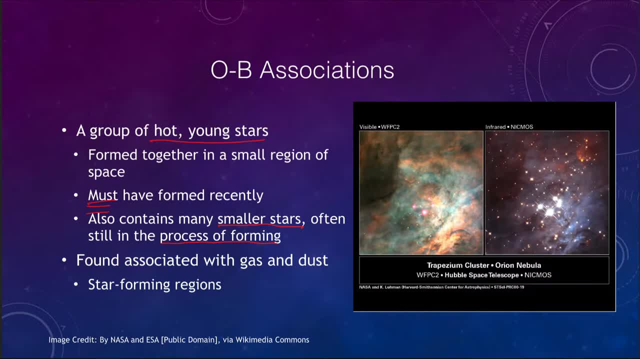 stars which are still in the process of forming. Just as a star goes through its life faster at a higher mass, it also forms faster at a higher mass. So when stars begin to form from a cloud of gas and dust in space, the first ones will be the most massive stars. 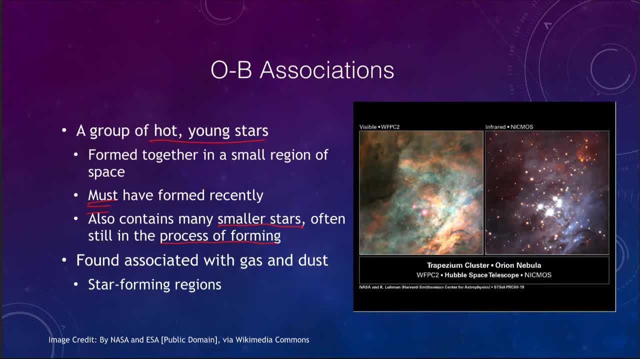 will form first And the low mass stars will take a much longer time. So these ones, these OB associations, are associated with star forming regions. Now let's look at how we can study stellar evolution in clusters like some of these, And how we can go about doing. that is, first of all, 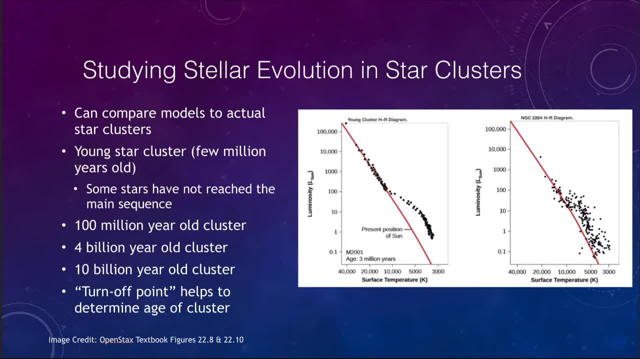 to look at the HR diagrams. What we can do is compare models to the actual star clusters So we can make a prediction as to how old a cluster should be and then how it should age over time. So as we look here, we see the young cluster HR diagram. 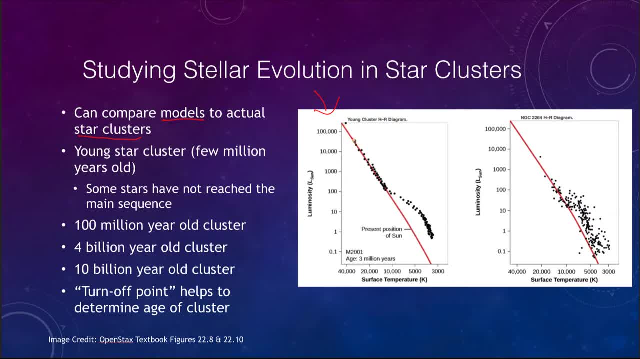 So what should a very young cluster look like? Well, it should have stars on the main sequence up here and it should have these lower mass stars still in the process of forming. These are ones that are slowly moving towards the main sequence. When we look at an actual HR diagram of a young cluster, 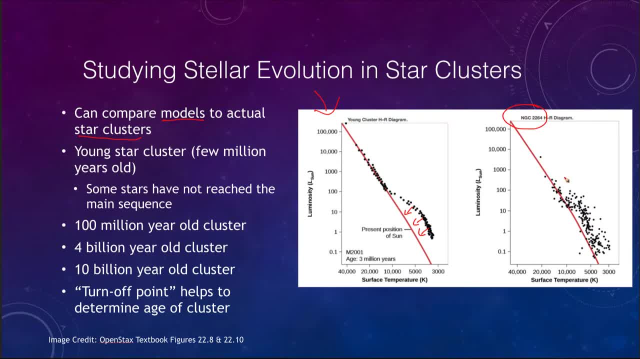 in this case NGC 2264,, we see something very similar. The higher mass stars are on the main sequence up here and there are low mass stars still forming. The higher mass stars are still moving down here. Now there is a difference in the amount of spread here. 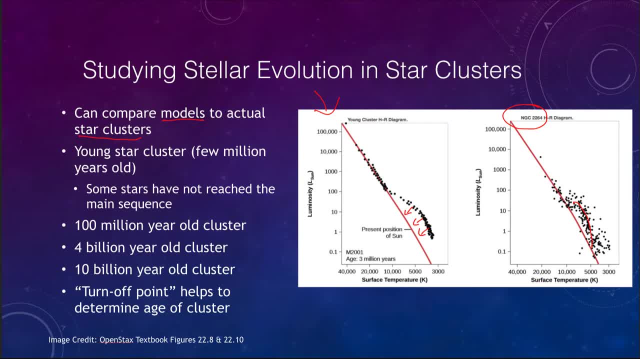 meaning that maybe these stars didn't all start forming at exactly the same time as they did in the model, and that some of them formed a little earlier and some of them formed a little later. So some of them are still in a little wider range. 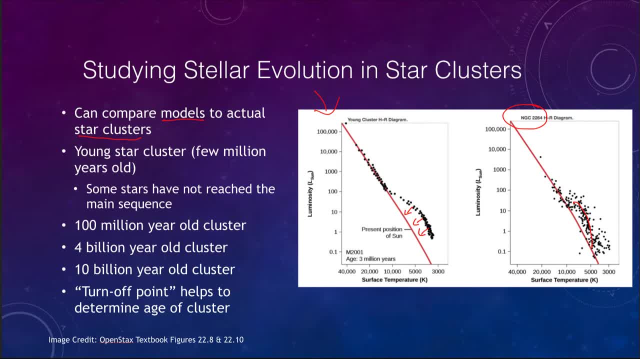 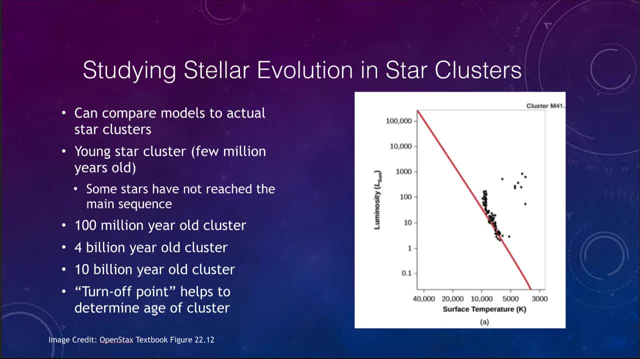 reaching down to the edge here. Now we can look at older clusters as well. So let's look at a slightly older cluster. This is a cluster at about 100 million years old, And at that age what we begin to see is that stars have now reached the main sequence. 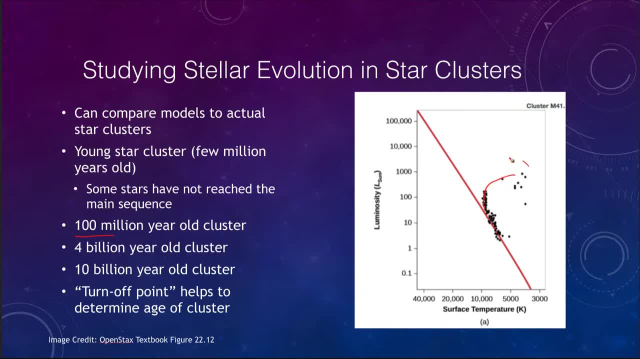 but stars up in the upper part are actually evolving off and are becoming red giant stars. So they have evolved off the main sequence and become red giants. So these are not stars that are forming as they were in the first slide. These are actually stars that are forming. 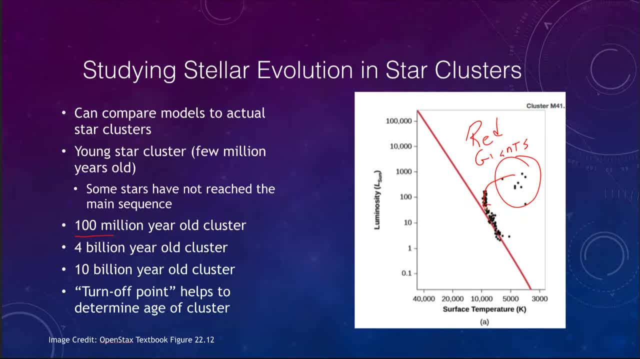 So these are not stars that are forming, as they were in the first slide. These are actually ones that are moving off And, if you notice, what we have here is what we'd call the turnoff point, the point at which stars are beginning to leave the main sequence. 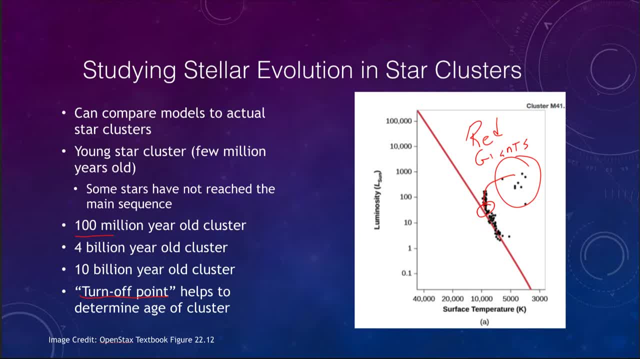 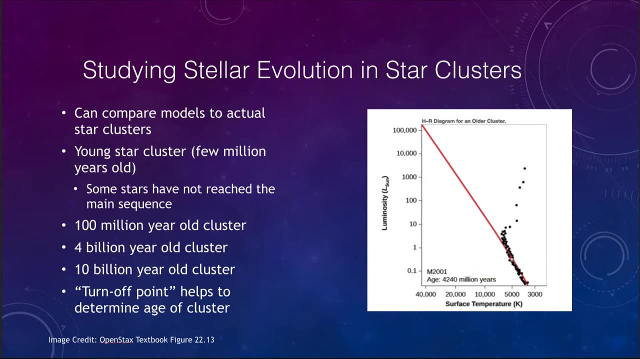 That is a way to be able to determine the ages of these clusters by looking at what that turnoff point is. A slightly older cluster would have again even more stars on the main sequence. All the stars have reached the main sequence down on the lower portion now. 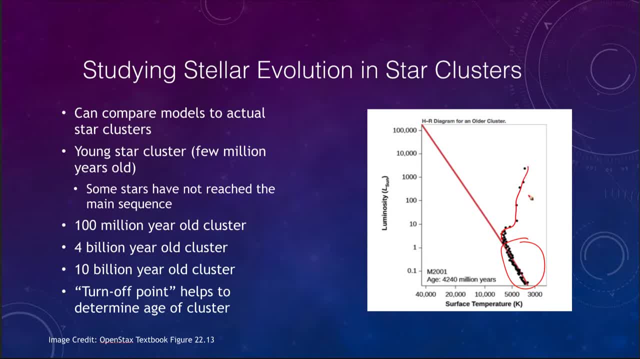 but all the other stars are starting to evolve off. There are no stars on the upper main sequence. They are gone. They have all gone through their lives and there are none left to be present at this point in this. So this is a cluster that is about 4 billion years old. 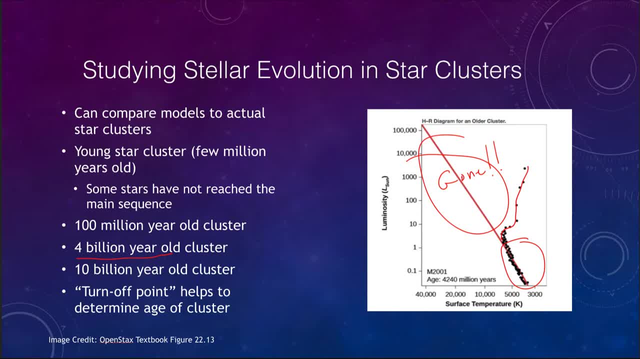 about the age of the sun- a little bit younger than the sun, but about that age. So stars are going to evolve, The stars in this region, the star like the sun, would be just getting ready to make its evolution off of the main sequence. 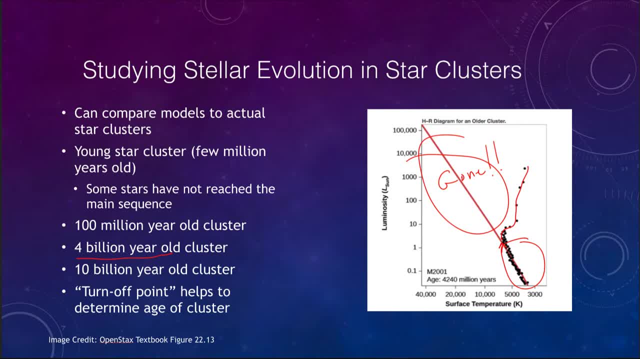 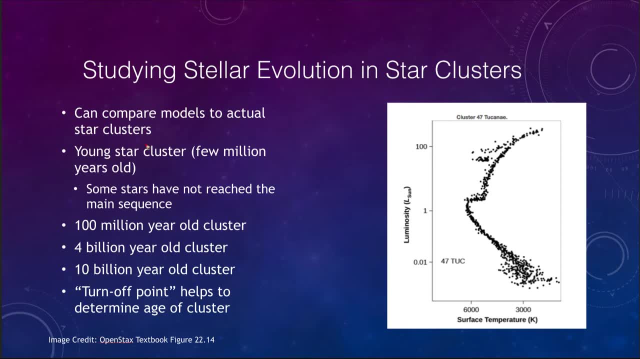 Now we can also look at a very old cluster, And let's take a look at one of those. And this is a cluster. This is an example of a globular cluster And what we see in these. this is about a 10 billion year. 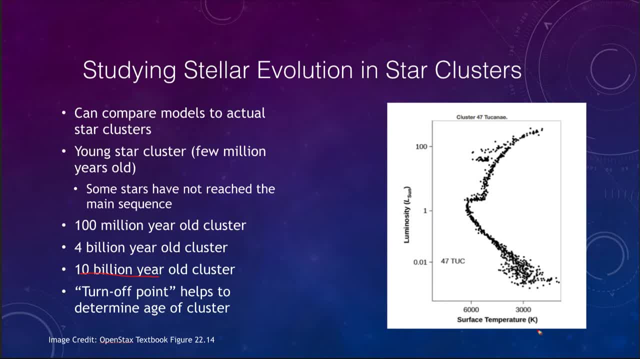 old cluster And now we start to see a lot of features appearing. Here is the main sequence, So the stars are that way, and here we see some of the stars that are going to evolve off of the main sequence. So these are the craters. 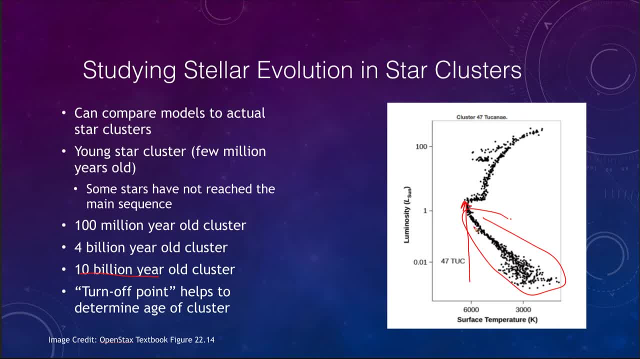 And what we're seeing here is the stars growing up here. so some of the stars are that way And we can also see some of these lines. So if we take this star here, these lines are moving off this line from here, over the edge of it, and we can see that it's. 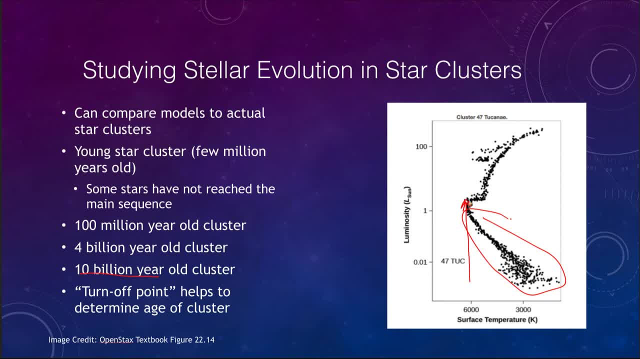 just like this, where it was when the sun began to evolve and develop These lines. these lines need to move off of the main sequence. So this is just a DNA sequence here, And the other thing as well. the surface of this is just like: 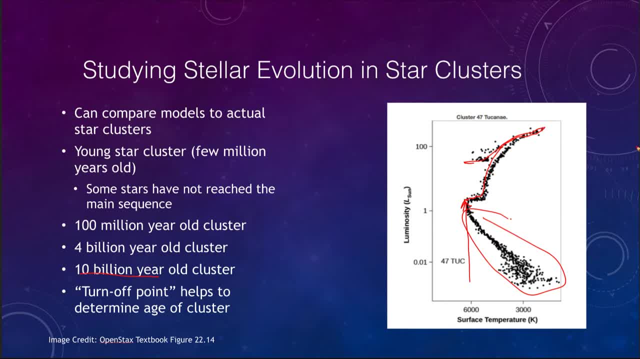 this area up here, come back down over here, So we can see that as the stars, slightly more massive than the sun, have already gone through, already in the process of going through their lives. But this turn off point again is what is important, because that allows us to determine. 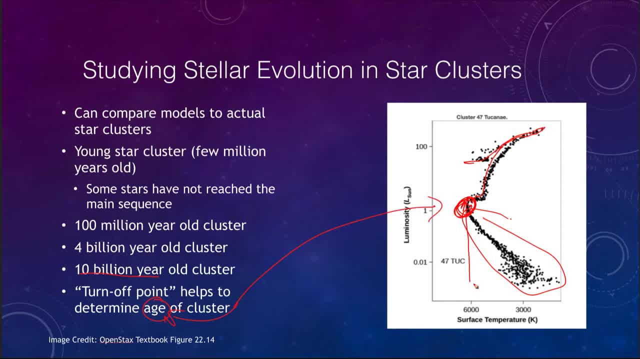 the age of the cluster Where this point happens to occur. what type of star is just turning off? the main sequence gives us the age, And we can then learn how old a cluster is. So let's get an idea of how old these clusters are. 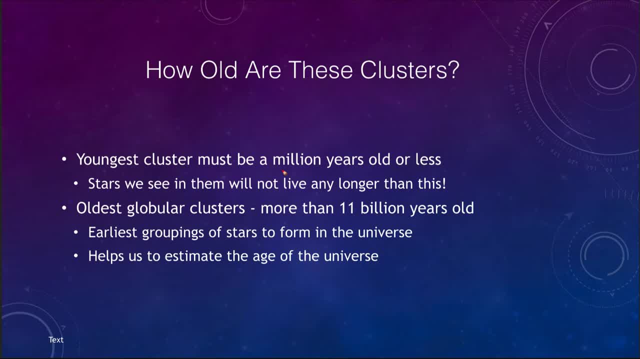 What do we know about some of these? The various youngest clusters must be a million years old or less. That's because stars that we see there will not live any longer. If these clusters were 2 million years old, those stars could not be there anymore. 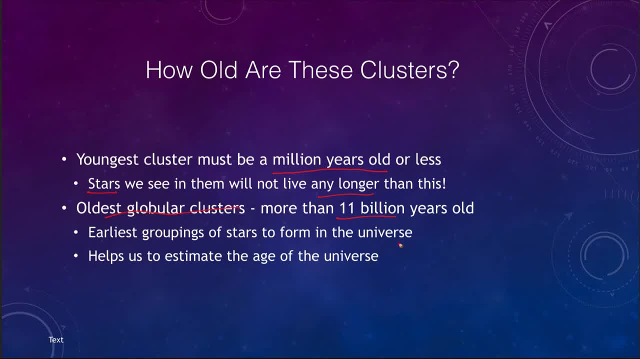 The oldest globular clusters we find more than 11 billion years old. These were some of the earliest groupings that formed in the history of the universe and can give us an estimate of the age of the universe, because certainly the universe cannot be younger than the oldest stars in it. 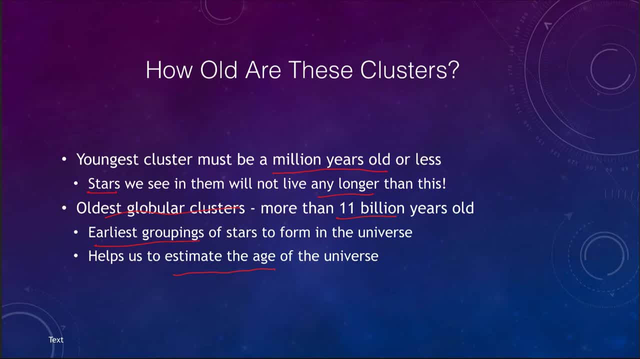 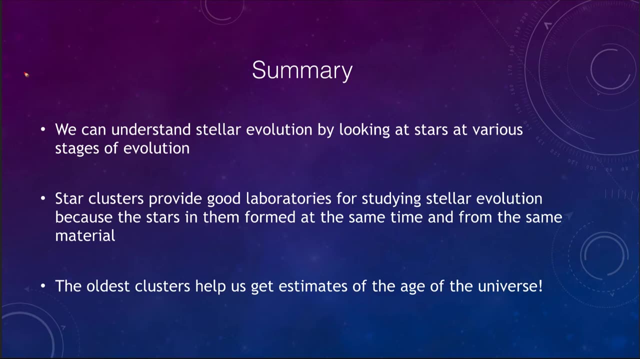 The universe has to be at least as old as the oldest stars, because stars could not have formed before the universe. So let's finish up here, as we do with our summary, And what we've looked at this time is that, first of all, we have a way of understanding.